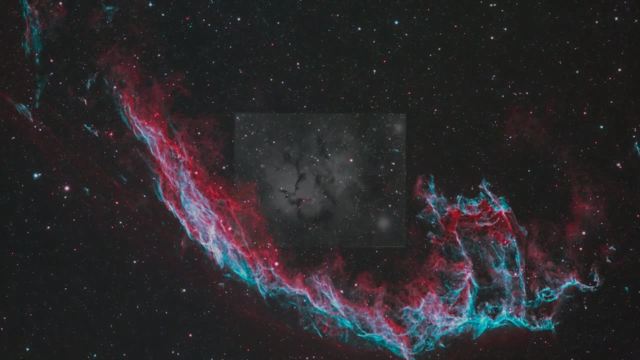 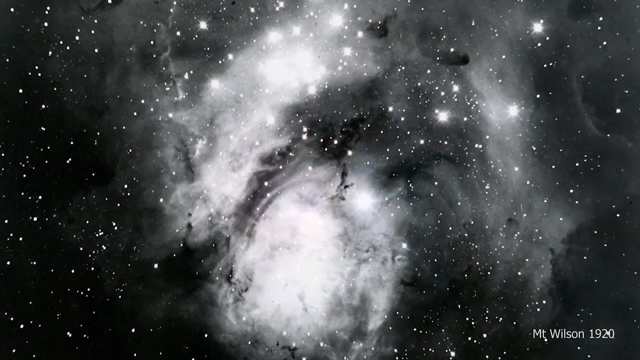 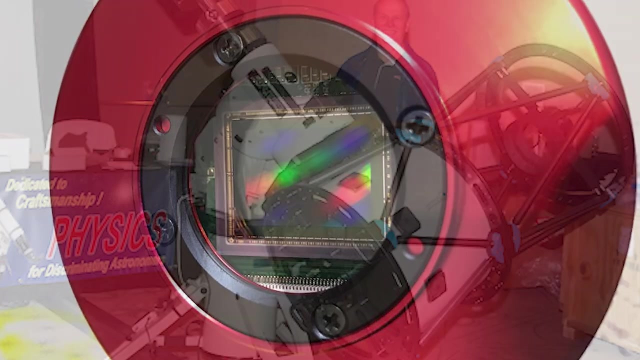 Comparing images produced by the best scientific teams and cutting-edge equipment from 50 to 100 years ago, they are far surpassed in clarity and depth by today's amateur imagers. even with modest budgets, Advances in sensor technology, precision, tracking, optics and affordability have all 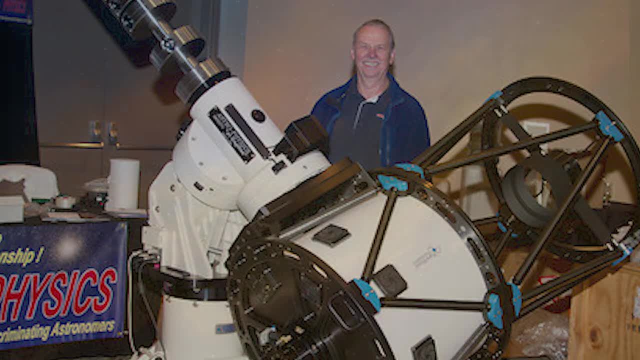 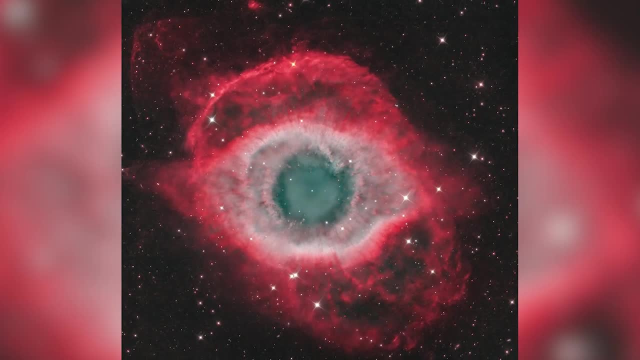 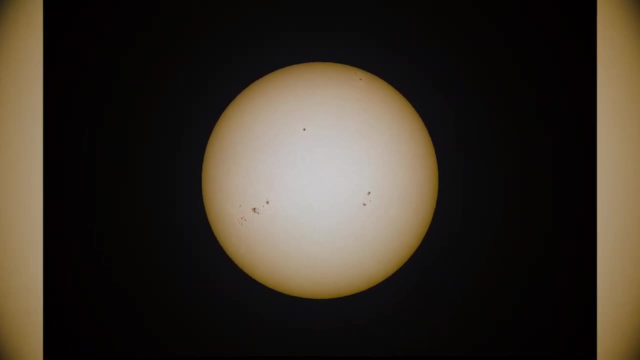 contributed to these astonishing improvements. Precision tracking, specifically, is one of the pillars for these advancements. Simply put, if the target doesn't stay precisely still, it won't matter how good your camera or optics are. Precision tracking allows us to take sharper images for longer periods of time. 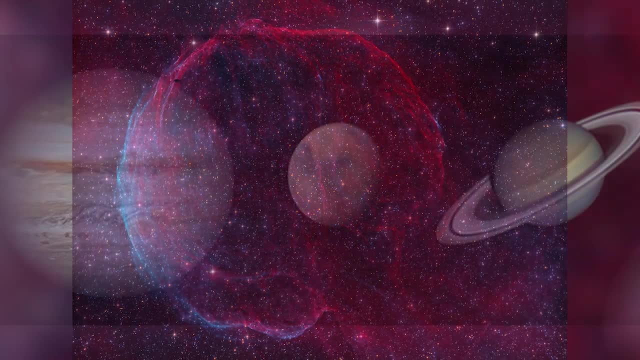 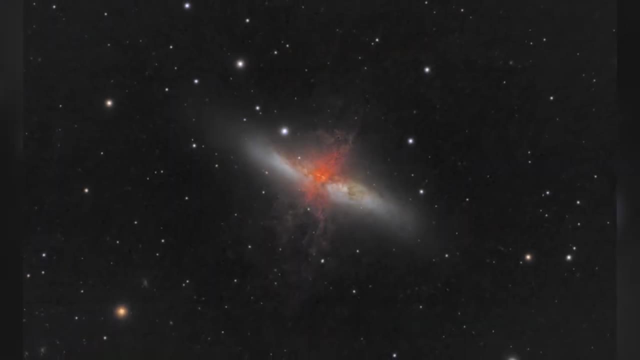 and return to targets, with repeatability for days, weeks, months and even years. But we humans, we are creatures of progress. We are always looking for ways to improve and make it better. We want our images to be closer, sharper, deeper and reveal more. 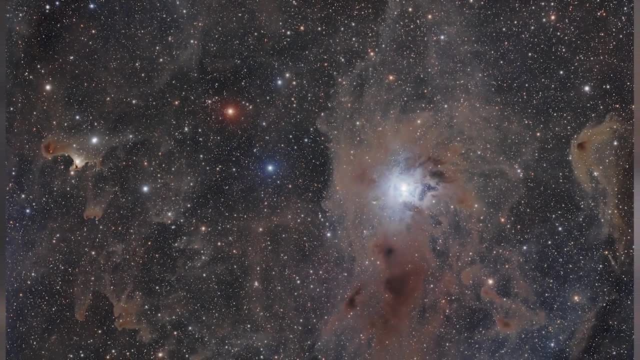 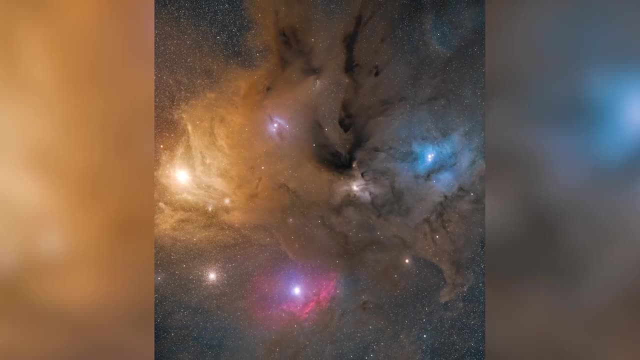 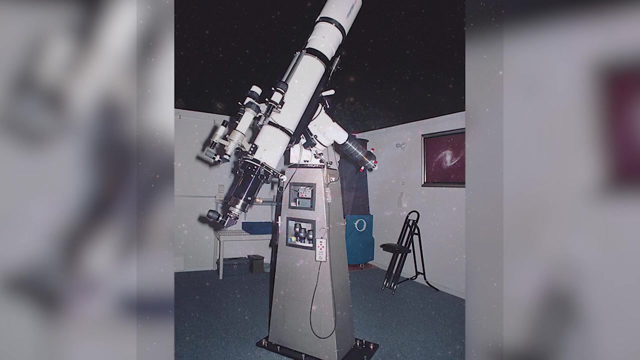 of the mysteries of the universe to our eyes. As we progress, it gets increasingly difficult to eke out performance improvements In order to take it to the next level. we are talking about improvements at the microscopic level, often fractional widths of a human hair- To make these types of advances with such precision? 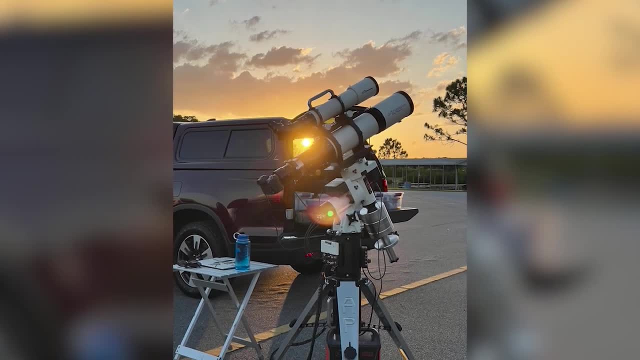 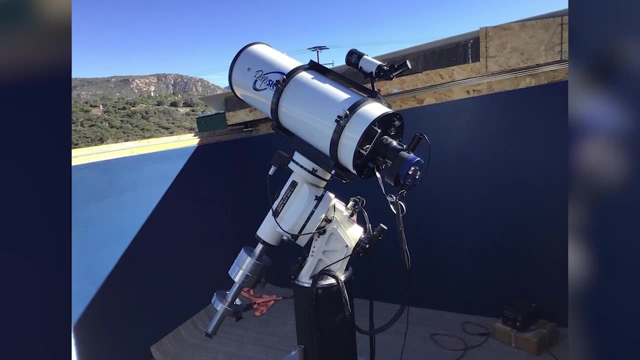 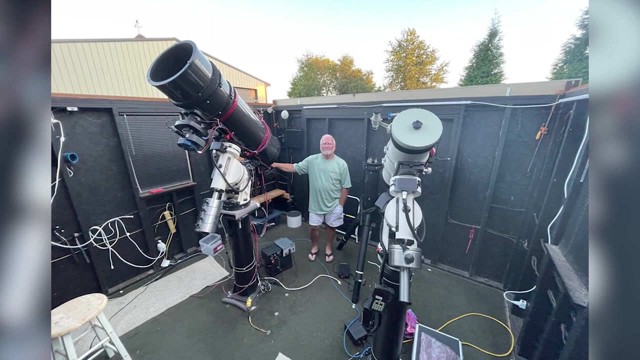 we can't simply use the same things as before and just do more of it. Measurable improvements come with new innovations in technology and software that build upon what we already have. Astrophysics already delivers best-in-class performance, but astrophysics also understands the relentless 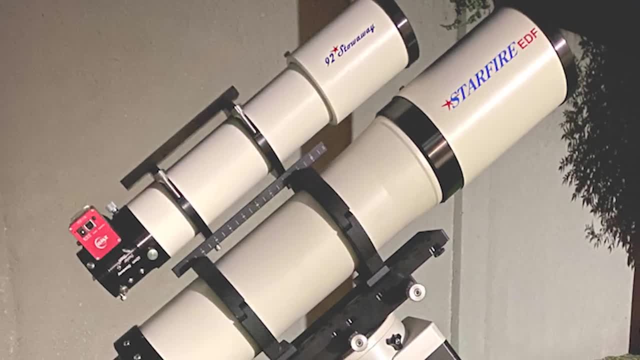 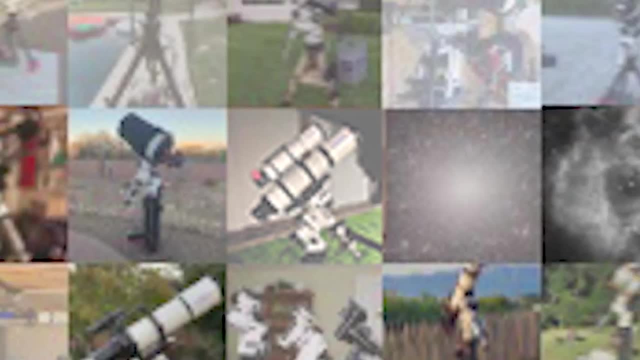 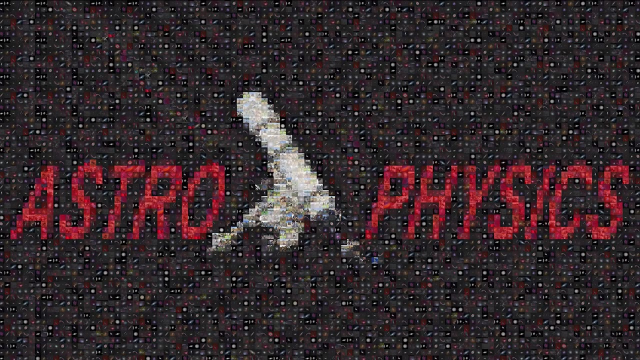 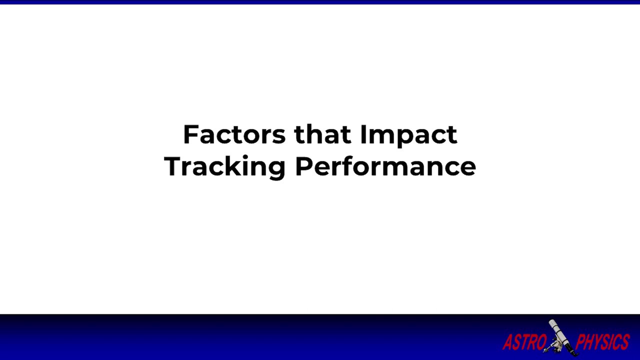 pursuit of this perfection. Astrophysics, introduction and ongoing refinement of absolute encoders and sky modeling continue to push the bar ever higher, and we will discuss the best use of these in the context of tracking improvements. Let's start by looking at some of the challenges we face in our quest for 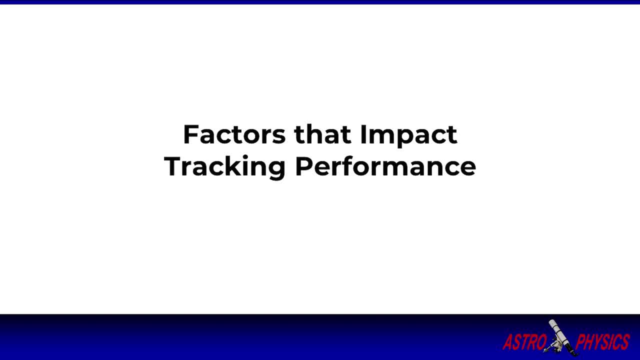 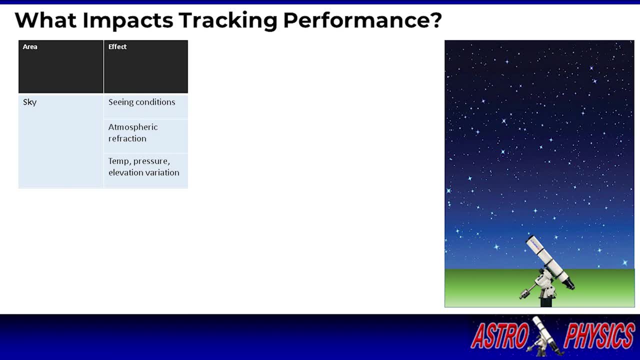 precision tracking. These problems are fairly universal and not specific to any mount conditions or technology. Until we can all afford space telescopes, the Earth's atmosphere creates issues for us. Seeing conditions are highly variable and contribute to apparent star motion distortion and generally just make things less sharp. 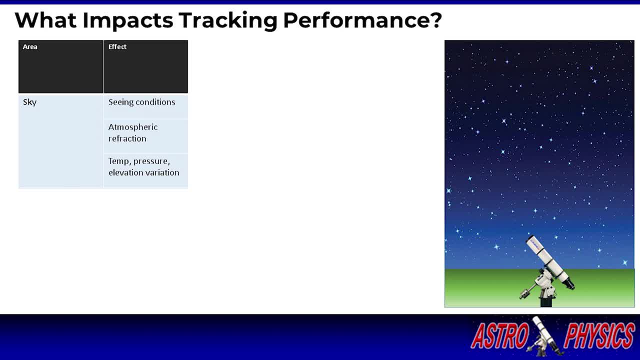 Atmospheric refraction. the bending of light as it travels through our atmosphere constantly changes our target's visual appearance, position and apparent motion. On top of this, variables in temperature, elevation and atmospheric pressure further compound these issues. Telescopes, image train assembly and their setup also create issues. Telescope tube materials and 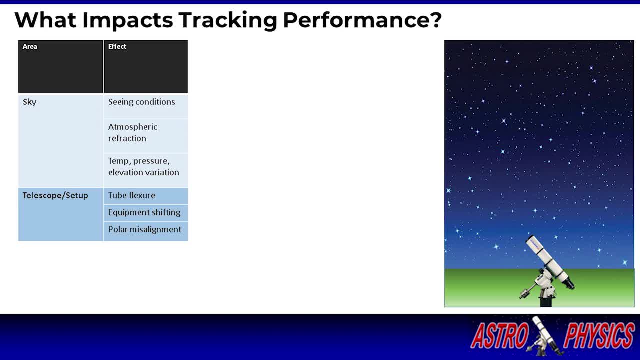 other components can and do flex with changes to sky position and temperature. Temperature and sky position changes can also cause shifting of equipment position and centers of gravity And polar alignment. inaccuracies and shifting can degrade tracking accuracy and will always be present to some degree, despite our heroic alignment efforts. 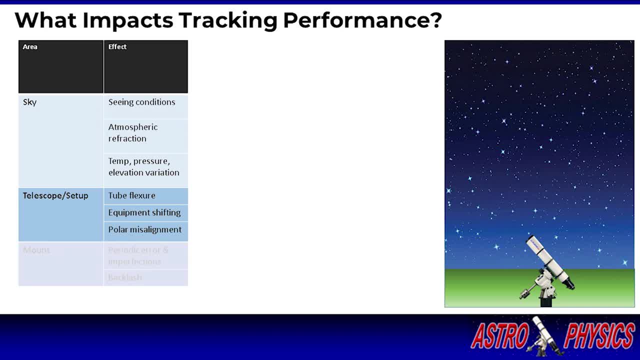 and the convenient and fantastic modern computer-based assistance. Finally, mounts bring their own challenges to the table. Minute imperfections in gears create tiny, repeatable errors known as periodic error. Other small imperfections in gearing, such as tooth imperfections, dirt in the gears and poorly 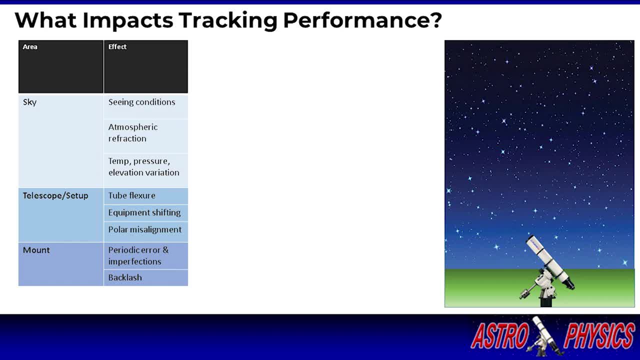 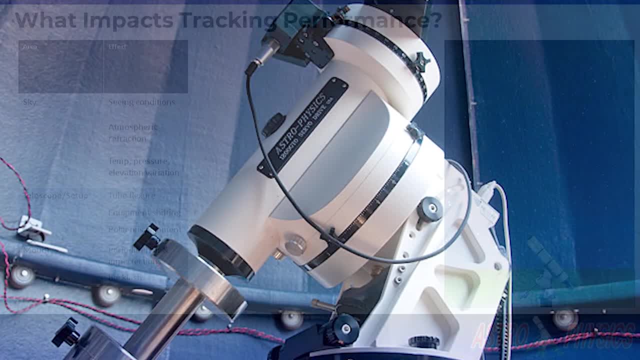 adjusted gear trains may contribute additional error. Backlash in the deck access can also add challenges when guiding. That's not to say all mounts are created equal. Premium mounts, such as astrophysics, are designed, machined and assembled with the tightest tolerances available to minimize 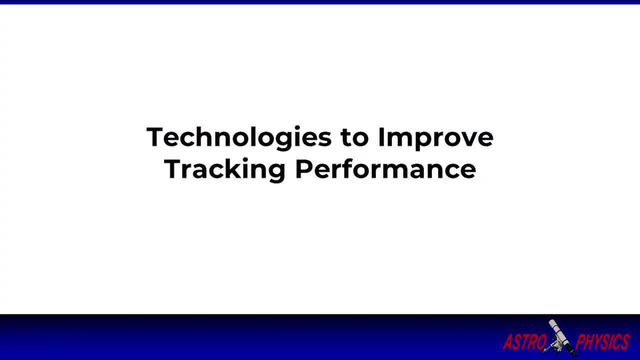 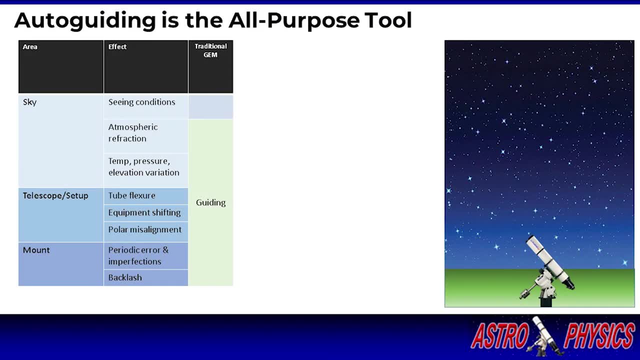 these effects. Now let's look at what technologies and approaches are available to address these potential image killers. The most traditional approach is using auto guiding to handle it all. As the guide star moves, auto guiding software evaluates its position and, if needed, 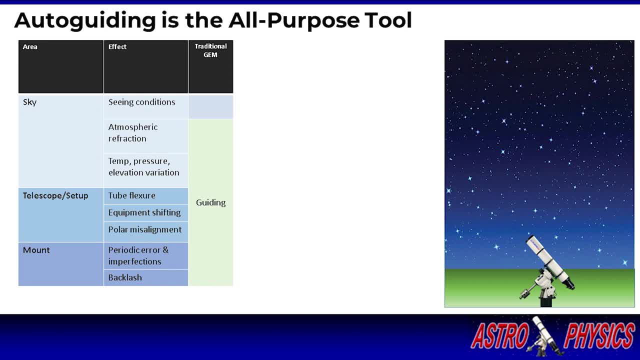 attempts to correct it using guide pulses and the resulting small mount movements. Periodic error correction, or PEC, has been around for a while and is a great technology to address the specific issues of periodic error and gearing imperfections, Using tools like PEMPro, which is the standard PEC. 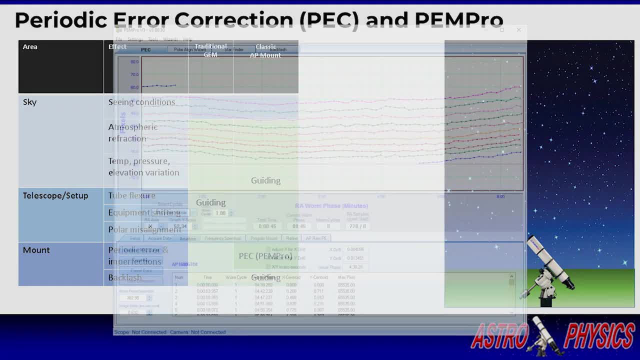 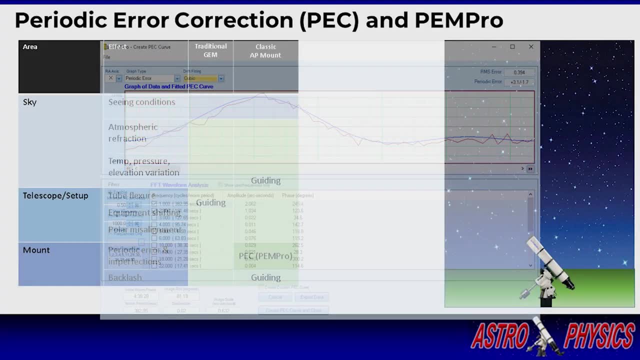 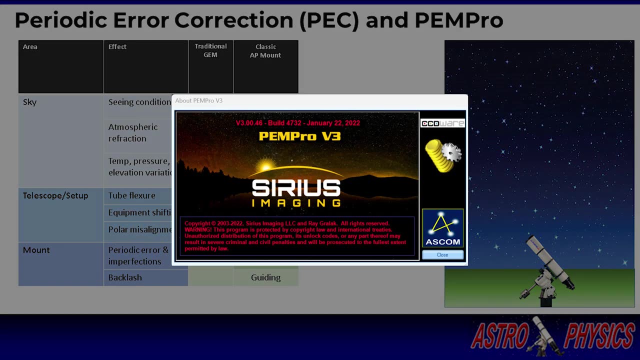 software for astrophysics mounts. these minute imperfections are captured during a training session, A correction curve is created and loaded into your mount, and these errors are then automatically removed during subsequent mount operation. with improved tracking, PEMPro is sophisticated enough to measure and apply these corrections at exactly the right time without 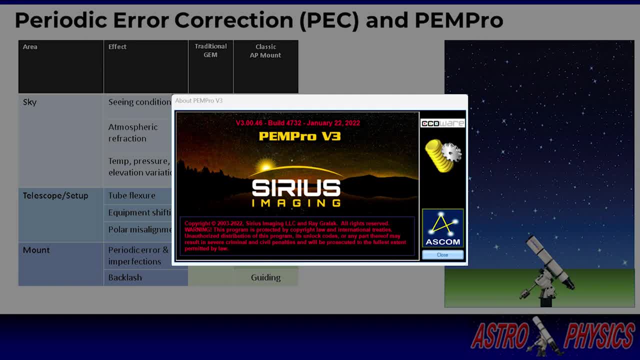 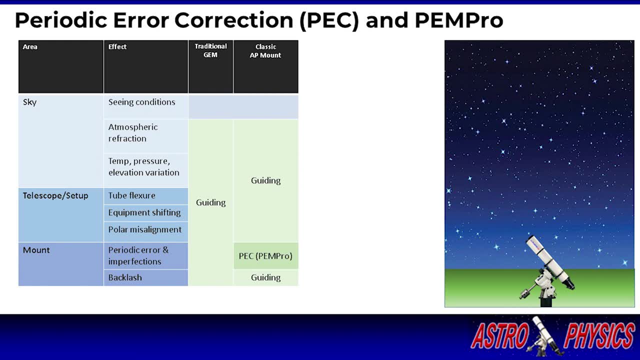 delay, so there's no driving by the rearview mirror effect. PEC does a great job at correcting for periodic error, but the other tracking challenges remain. Auto guiding in this example remains an important complex. PEMPro is a great tool to use for correcting for periodic error. 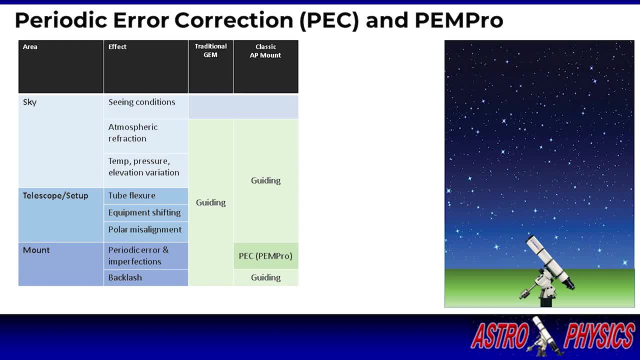 Auto guiding in this example remains an important complex. Auto guiding in this example remains an important, complex PEMPro is a great tool to use for correcting for periodic error. By removing periodic error, PEC also has the added benefit of improving auto guiding. It's a win-win. 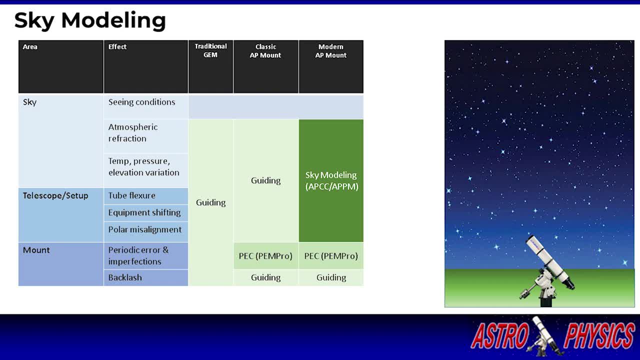 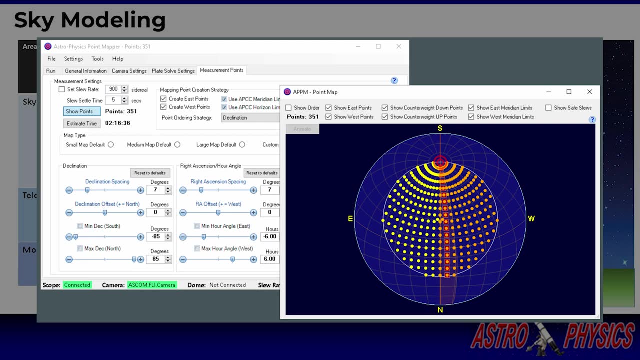 SkyModeling is a powerful and relatively recent software addition that can counteract the adverse effects of atmospheric refraction, temperature pressure and elevation changes. on tracking To use SkyModeling, a modeling run is completed in advance using the APPM tool, which is part of APC. 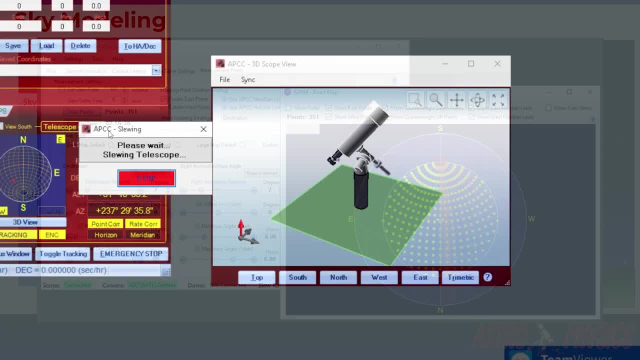 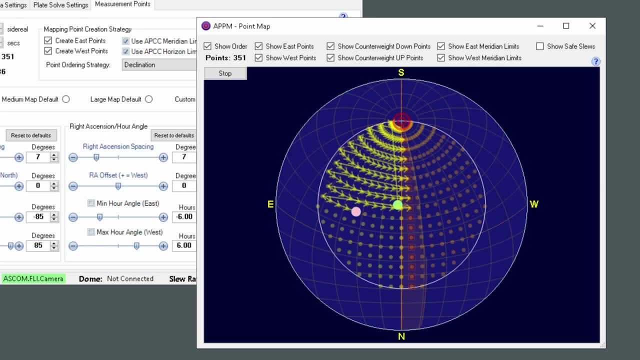 To use SkyModeling. a modeling run is completed in advance using the APPM tool, which is part of APC. The telescope slews to different parts of the sky where it measures and compares the expected sky position with the actual sky position. A typical run can consist of a few dozen or a few hundred. 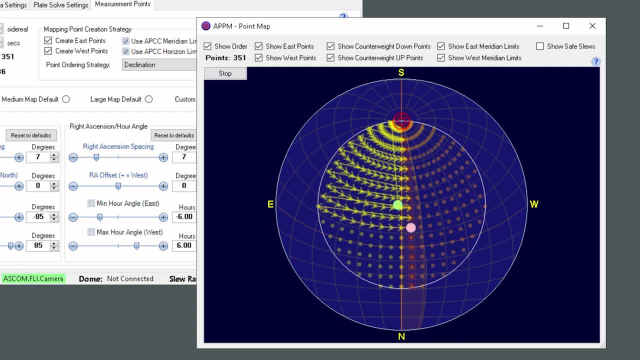 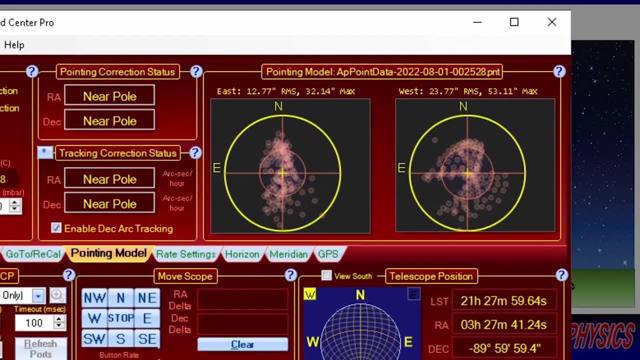 measurements across the sky. The results are then stored within APCC software, which then uses this information to refine tracking rates as the telescope moves through the sky or as conditions change. Again, this is a solution that proactively addresses these specific challenges, rather than. 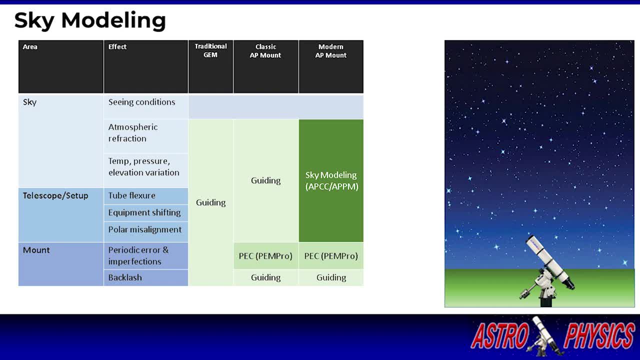 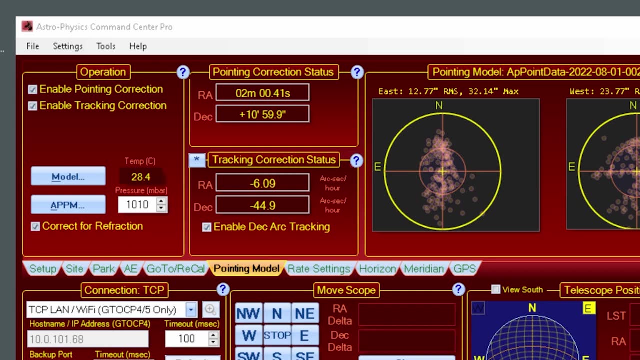 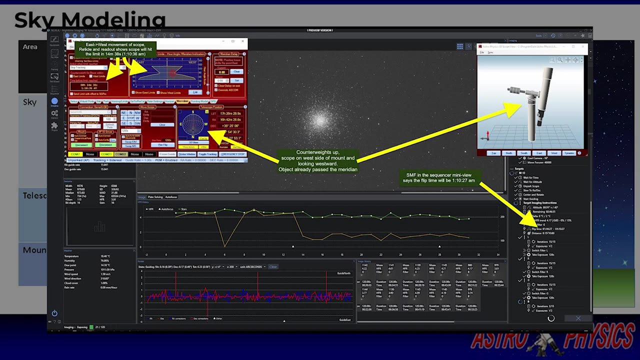 reacts to them- Another example of near real-time improvement. Since its introduction, SkyModeling in APCC has become increasingly sophisticated, with new, improved algorithms such as deck arc tracking to make tracking even more precise. Improved integration with third-party software such as NINA enable mobile imagers to build sky models on the fly for specific targets in just a few minutes. 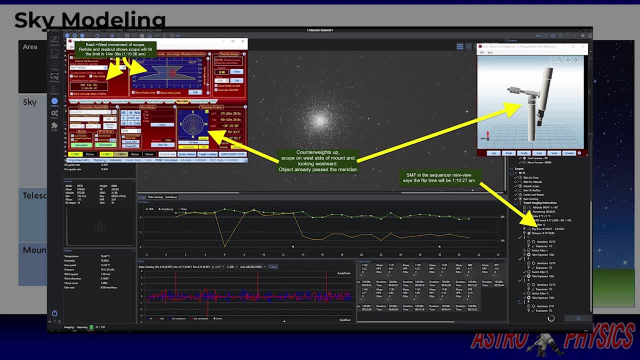 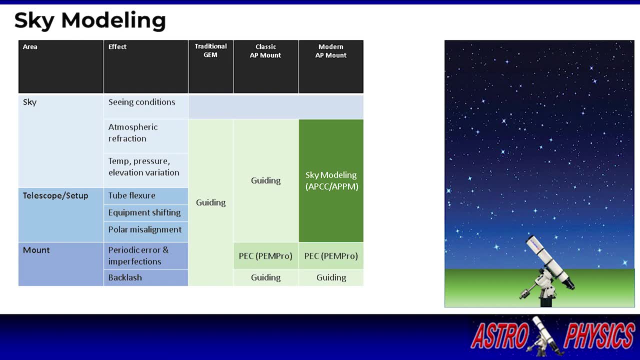 and can therefore take advantage of SkyModeling without a lot of upfront investment in time. As you can tell, SkyModeling excels at addressing specific atmospheric and condition-related challenges, but doesn't focus on the other areas, such as periodic error. You can therefore see: 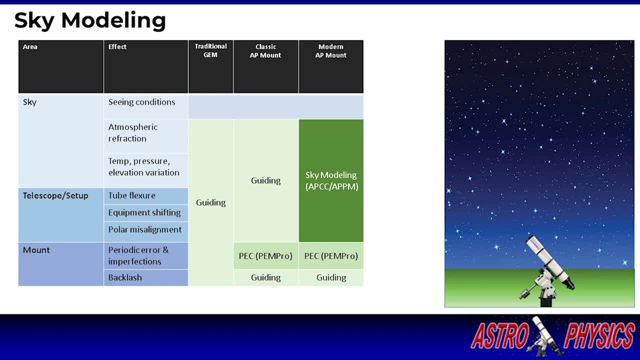 combining SkyModeling with PEC can enhance tracking across a broad range of problems And, as we can also see, auto-guiding still plays a role for the remaining issues. Our picture evolves even more with the addition of absolute encoders. Absolute encoders is an 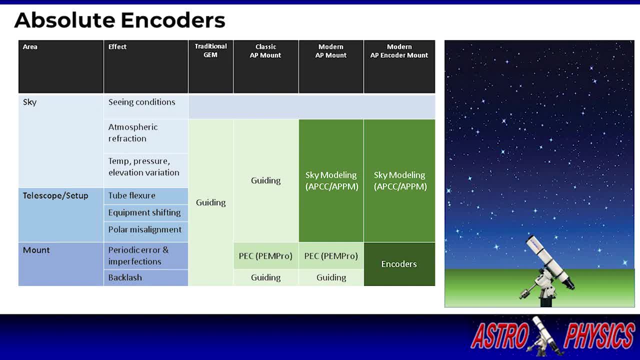 extremely powerful technology for precision tracking. These hardware encoders are affixed directly on each axis to measure expected position versus actual position and the resulting encoder corrections effectively eliminate the minute mount gearing errors. Unlike PEC, encoders also address gear backlash, in addition to periodic error and mechanical imperfections. Encoder 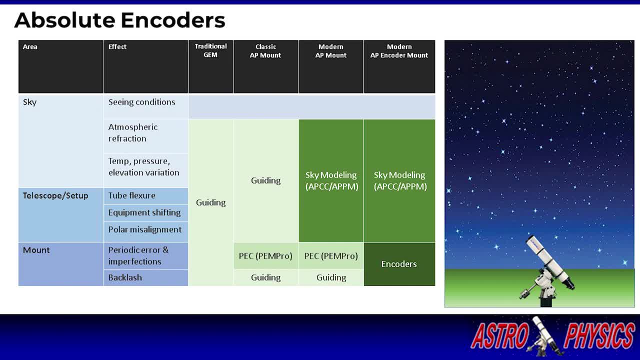 monitoring and the corrections here are so close to the source and so fast that they are effectively real-time, About the closest thing to achieving a theoretically perfect mechanical mount. Not only do these two technologies work well together, but absolute encoders also improve the accuracy of SkyModeling, So in this case the total performance is greater than the sum. 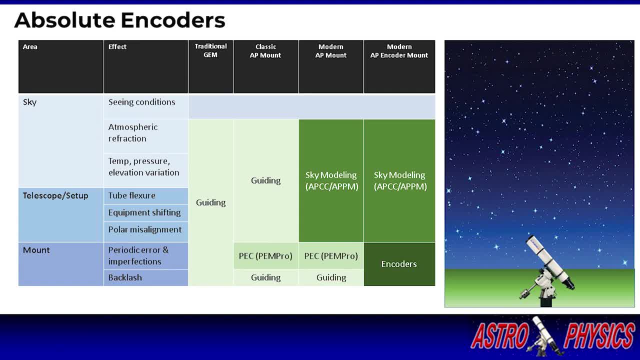 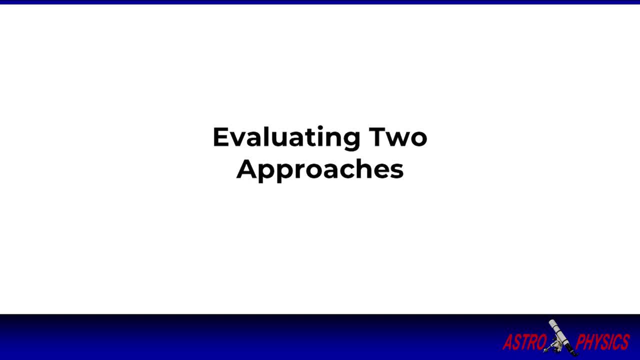 of the parts Combined with SkyModeling. now our approach has improved considerably. Now let's back up and look at a couple of obvious questions regarding what's the best tool or tools for the job. First is a guiding only approach, If guiding covers it all. 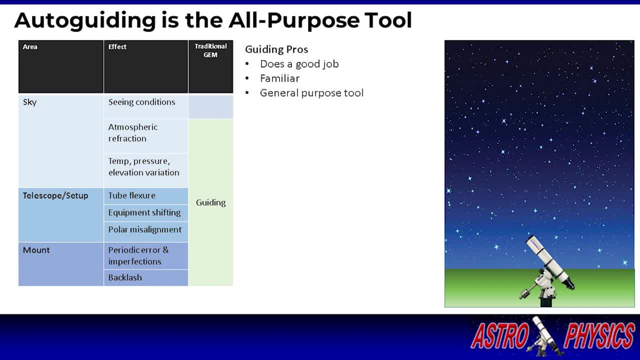 why not stop here and just auto guide? It's a great question, since guiding is familiar to many and can produce good results. However, auto guiding is a pretty coarse tool and may not be the best option in all situations. Auto guiding also comes with its own trade-offs and drawbacks. It's 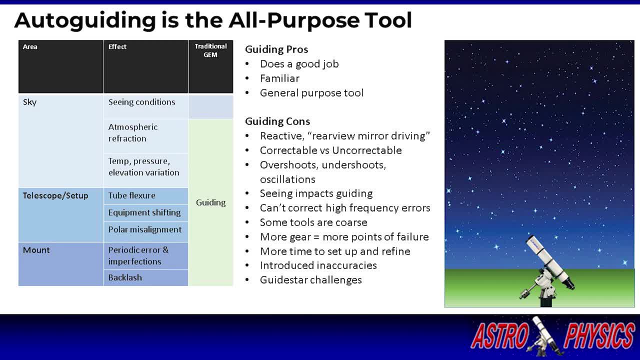 reactive. It corrects once the problem is measured, so the corrections will always be after the fact. It's like seeing a stop sign in your rear view mirror and then applying the brakes. Auto guiding can't distinguish between things that should be corrected, like drift, versus things that can't. 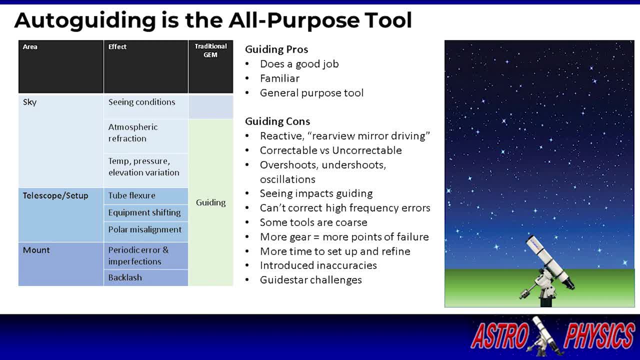 be corrected, such as seeing. So it can't precisely attenuate the amount of correction. Guiding can also introduce its own errors, such as pulse guiding overshoots under corrections and, extreme cases, oscillations. Poor sky conditions can further degrade guiding performance. There are 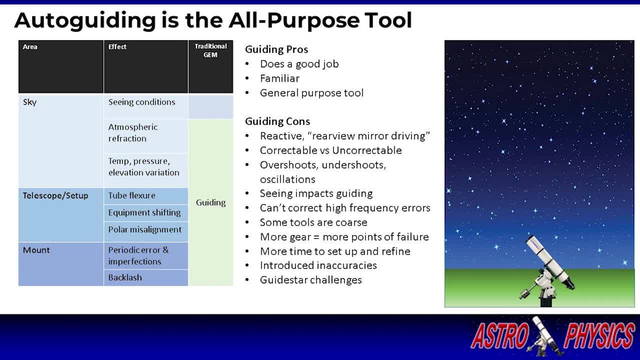 also some things that can't be addressed with auto guiding, such as higher frequency errors. Auto guiding software may not be flexible enough to account for changing conditions. For example, a single backlash compensation value may become less accurate with changes to the mount's sky position, And a lot of new things can and will go wrong when adding an. 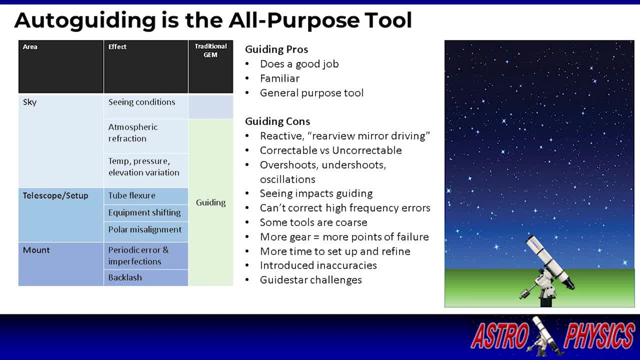 additional camera optics and software for auto guiding. The additional equipment, such as a separate guide scope, off-access guider guide camera, mean more potential points of failure. There is the added time and overhead for setup, calibration, dithering, settling rotator requirements and a lot more settings to 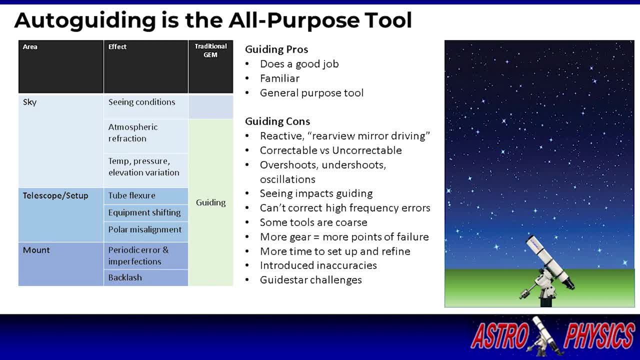 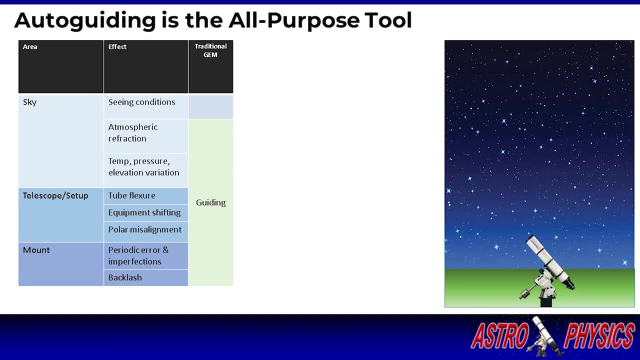 fine-tune. Auto guiding software has limitations as well. Oversampled stars can create centroid calculation issues, backlash compensation may not be sufficient or even available, and you may not always get good, reliable guide stars where and when you need them. So the message here is not that auto guiding is bad. 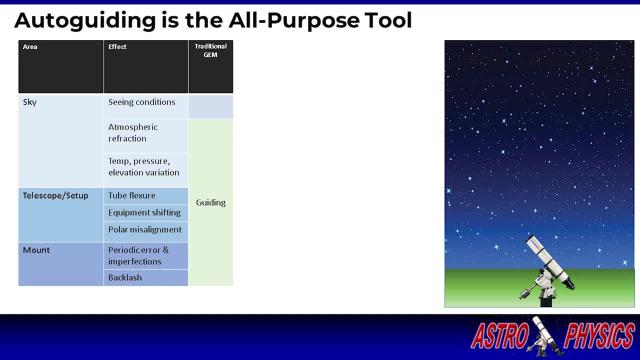 it's just that. as a course, all-purpose tool, it comes with trade-offs. In some circumstances it may be all that's needed, But in many situations and conditions there are other tools that can do a better job addressing specific types of concerns, and can do it with fewer added drawbacks. 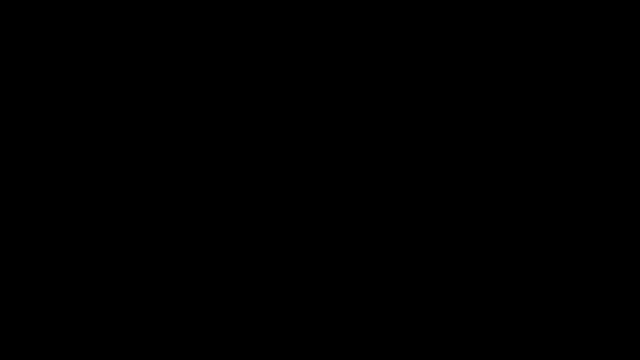 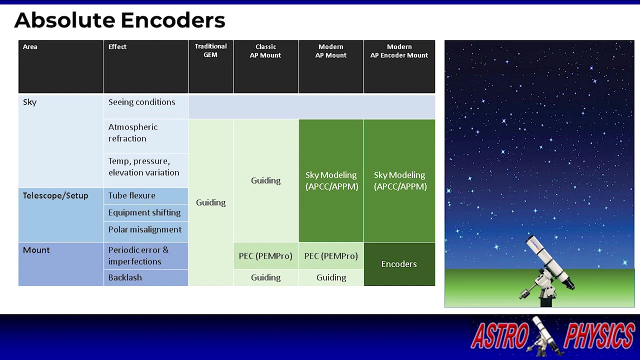 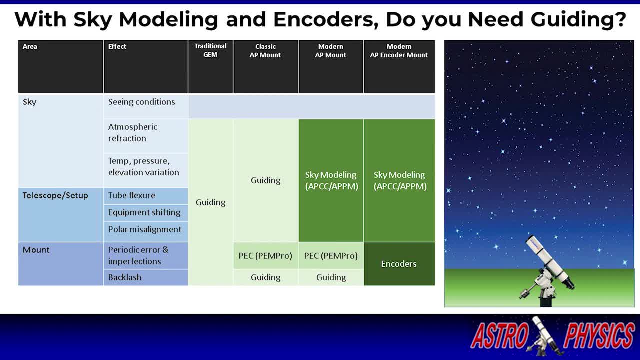 then how do we do it If we have absolute encoders and sky modeling that don't work? do we even need guiding? Again, a great question, because on the face of it, the answer would appear to be no, And in many cases, precision, unguided imaging is now possible. 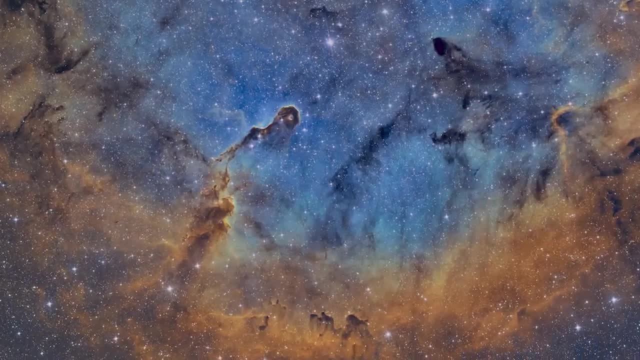 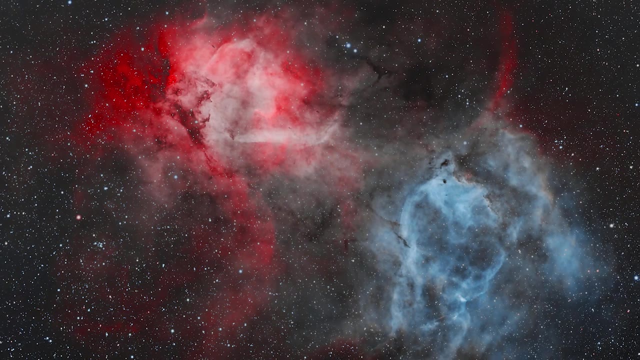 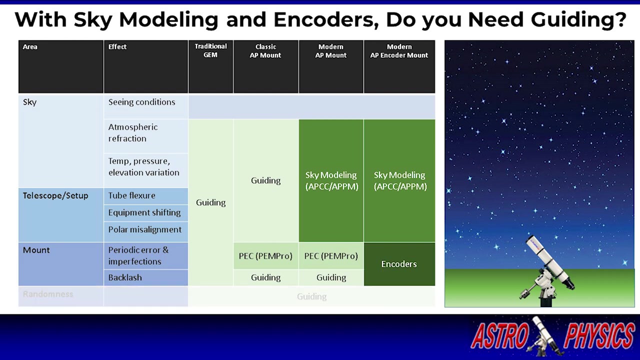 and practical. Many astrophysics customers today are doing unguided imaging and producing exceptional results, and often point out the ease of setup and use. It's just so simple and the results can be so good. So in this scenario, is there a role for auto guiding to play? The answer can be yes. The reason is: 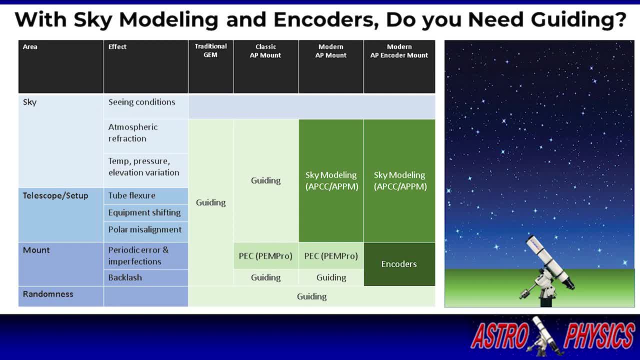 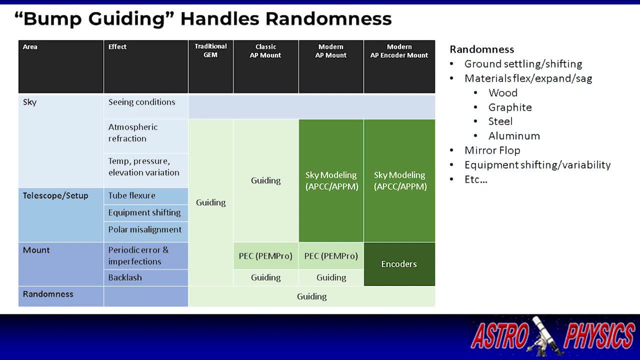 there will always be some amount of randomness and variability that just can't be predicted or modeled. These are things like ground settling materials, flexing and expanding- that include wood, graphite and aluminum- mirror, flop equipment. shifting and variability- There's just too many. 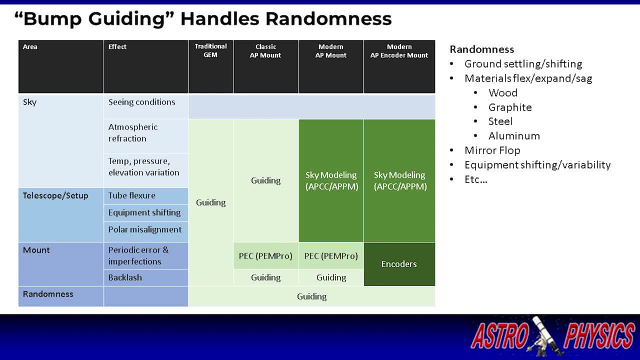 things here to list. Adding a gentle, catch-all type of auto guiding, also known as bump guiding, help ensures that small things don't add up and degrade your tracking. However, it may also be that you're specifically trying to get the best out of what you're doing and you're not.